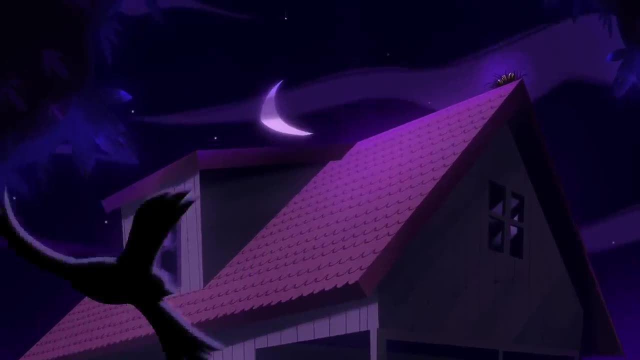 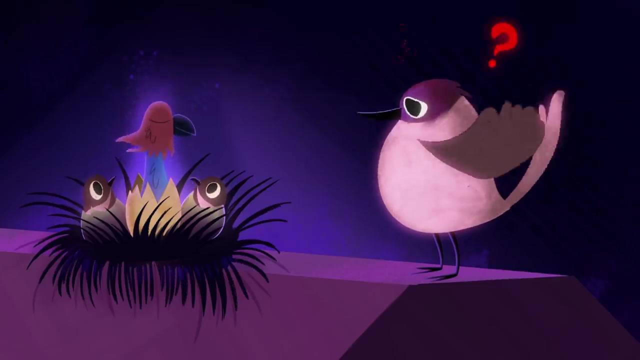 eggs and nestlings seems to depend on a few factors. Eastern Phoebes will accept a brown-headed cowbird's speckled egg into their nest, though theirs are pure white. The grey catbird, on the other hand, is an expert at rooting. 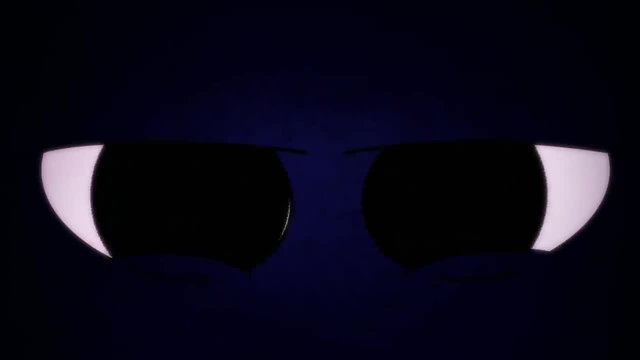 out the very same parasites. It memorizes what the first egg in its nest looks like, which is usually its own, And turns its egg into a hen egg. The first egg in the case of a nest is usually voracious, but these two are rather easy to bestow on their offspring. 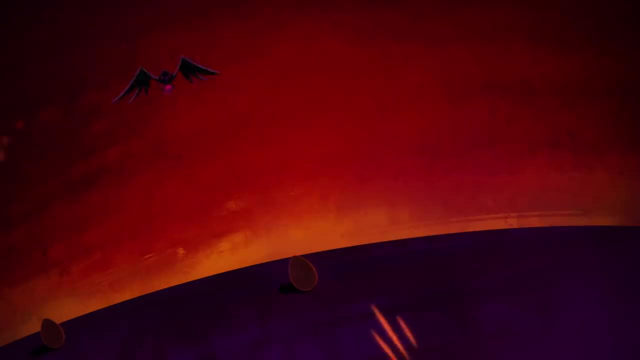 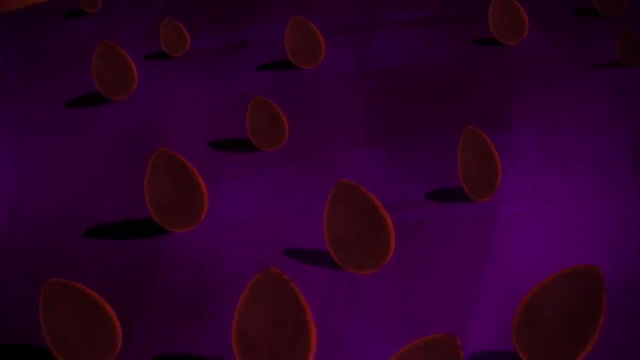 But in the rare cases of brood parasites, the egg is very common and the taste of brood tosses any aberrations. This retaliatory adaptation can fuel an evolutionary arms race, where brood parasites evolve eggs that closely mimic their hosts. 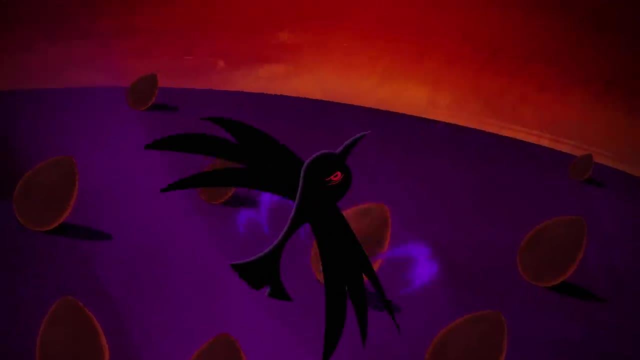 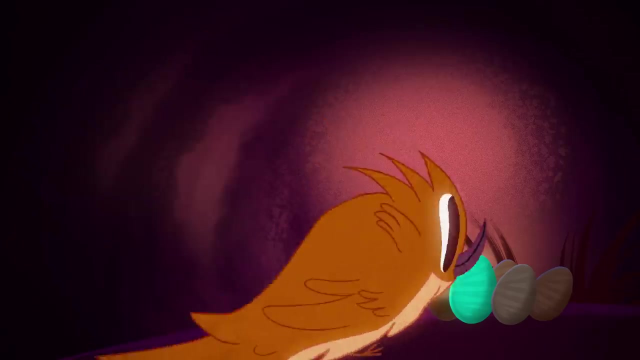 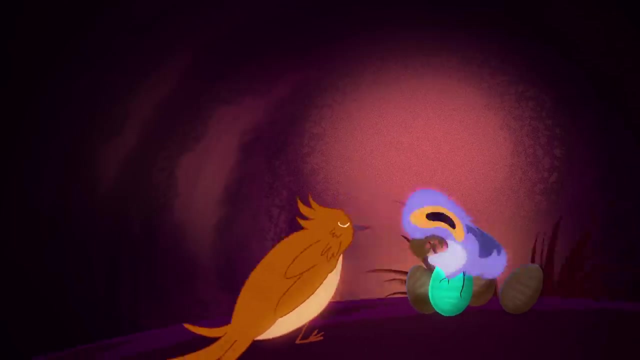 Interestingly, birds that do reject parasitic eggs are usually clueless when it comes to parasitic chicks. Reed warblers are good at ejecting poorly matching cuckoo eggs, but if one hatches in their nest, they'll care for it, even after it's grown six times their size. 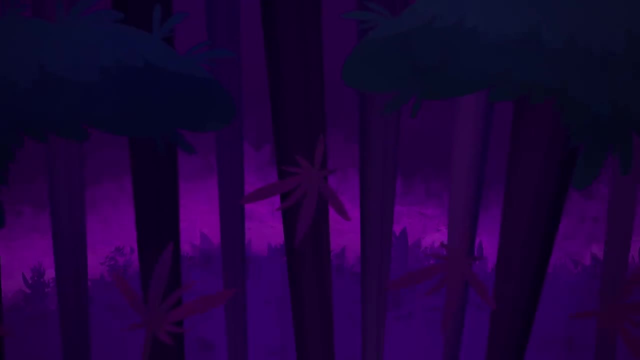 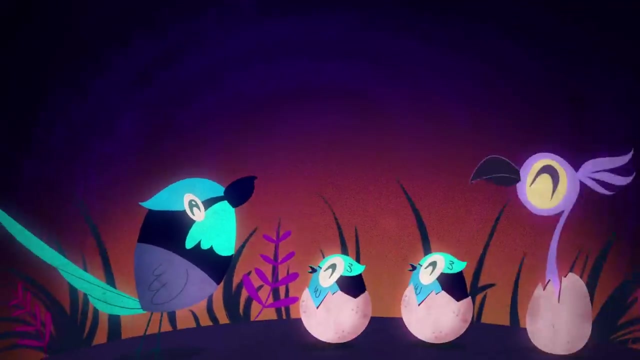 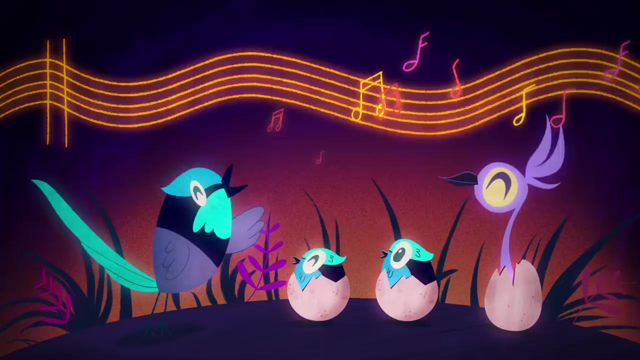 Though chick rejection is a rarer phenomenon, there are some noteworthy examples. While incubating its eggs, the Australian superb fairy wren sings to them, imparting a unique note that its chicks use as a kind of password: When a cuckoo is in the wren's nest, it hatches first and pushes the others out. but 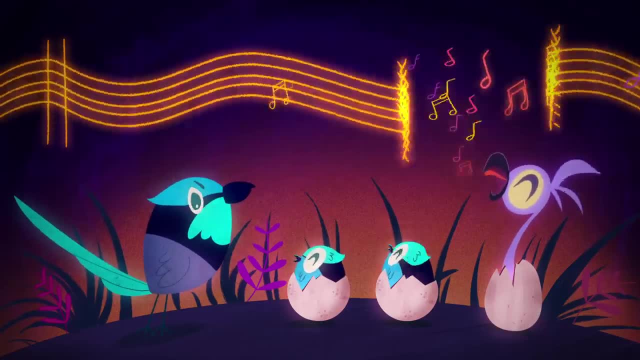 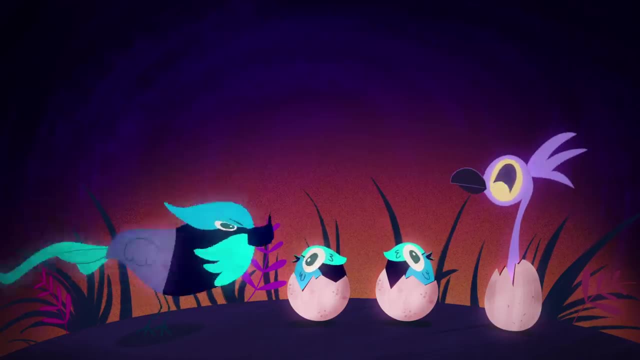 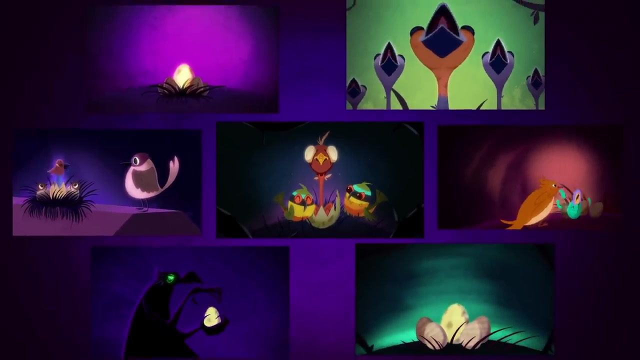 perhaps because it hatched sooner. the cuckoo chick wasn't able to learn the password, And so it doesn't croon the right begging call. At this point, the adults usually abandon their nest and start another Altogether. host species show a remarkable variety of responses. 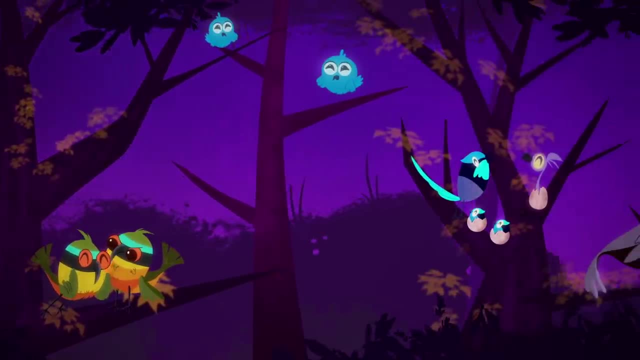 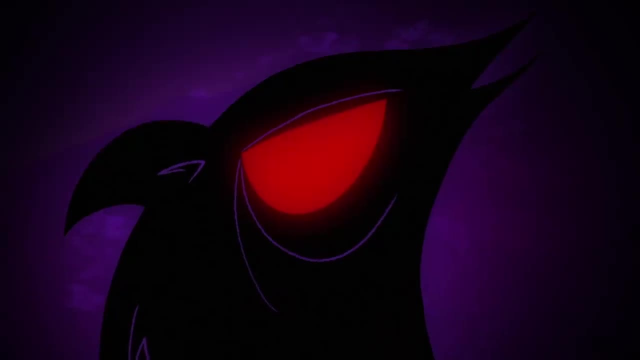 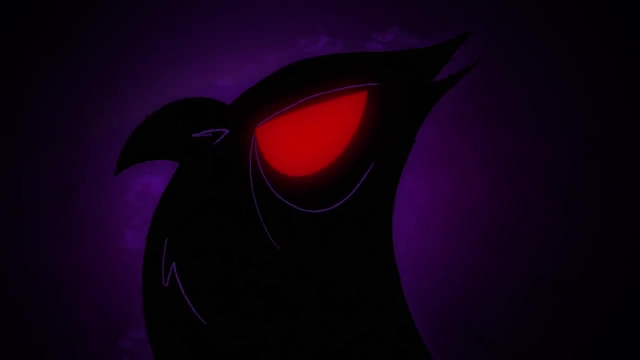 This seems to partially be a result of how long brood parasitism has been in their environment and thus how much time they've had to evolve suitable adaptations. In fact, studies have shown that those hosts that reject parasitic eggs less frequently can visually distinguish between their eggs and a brood. 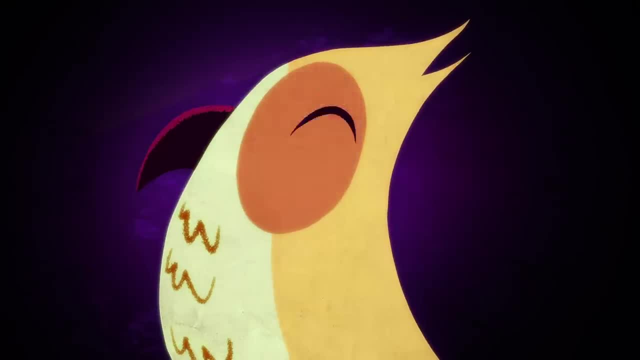 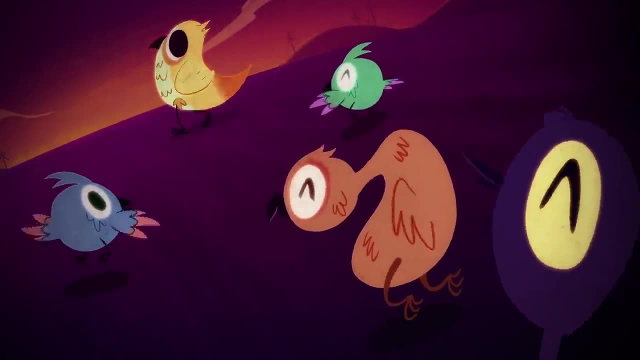 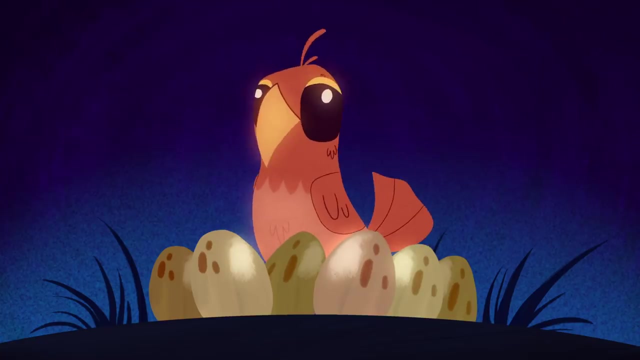 parasite's. They simply lack a response to the visual information. This is probably because, before brood parasitism appeared, responding would have likely had no adaptive value. And even when hosts do recognize a parasite, getting rid of it may not be the best option.